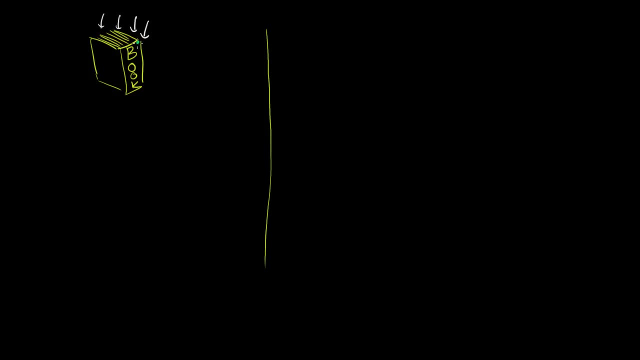 And so any point on this book- and we could pick any arbitrary point on this book- is going to be emitting light in a whole bunch of directions. So what I'm just going to do is pick two light rays that are being emitted from this point on the book. 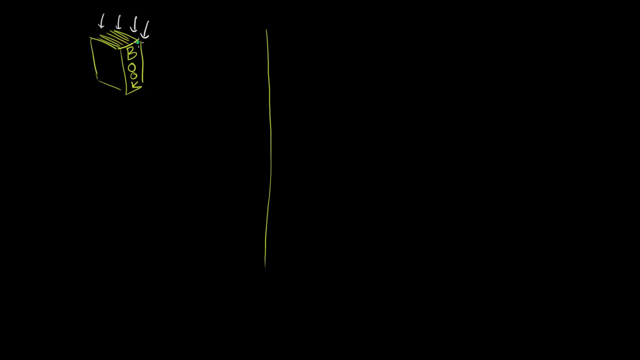 It'll be more than two, but this will help us understand what's going on here. So let me pick one light ray that goes like this: It's obviously not curving like that, So it goes like this and hits the mirror: Incident angle is equal to reflected angle. 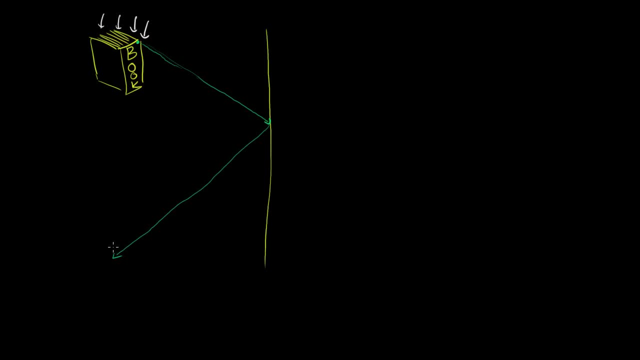 So it will reflect off at the same angle, just like that. And let me pick another point that is coming out radially from that same or another ray that is coming out radially from that same point, So it'll come out like that. 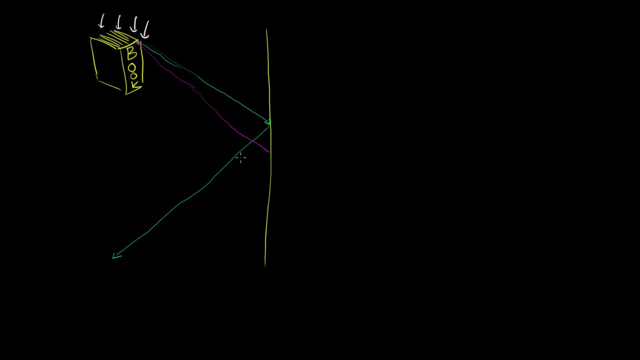 It will come out like that: It has a larger incident angle, so it'll have a larger reflected angle, just like that. And now let's think about what an observer: someone who has their eyeball right over here. So let's say, someone has their eyeball right over here. 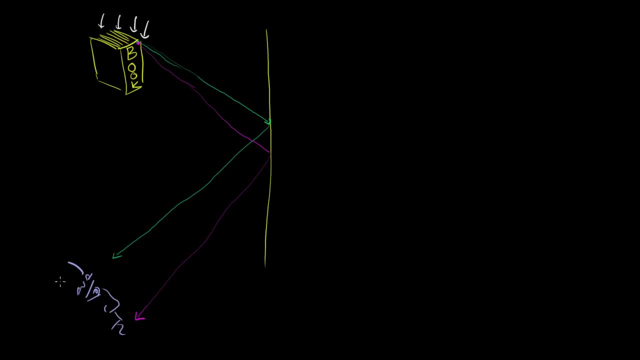 So let's think about what this person- let me draw their eyebrows so you get the general idea- Let's think about what this person right over here will actually see Now their eye and remember all of reality is really just a big simulation. 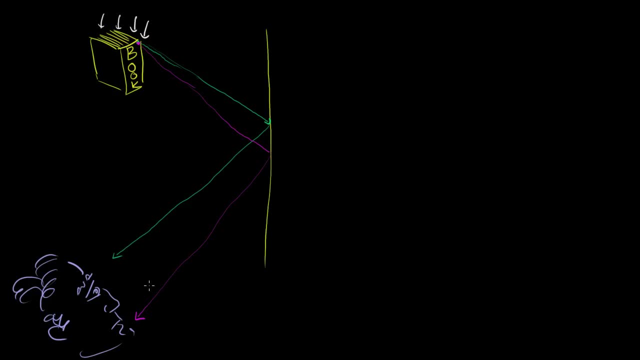 It's not going on in our brains. Now this person's eye is going to see these two light rays diverging from some common point. If you were to look straight at the book. or- let me just do another example- If someone were to just look at any arbitrary object, 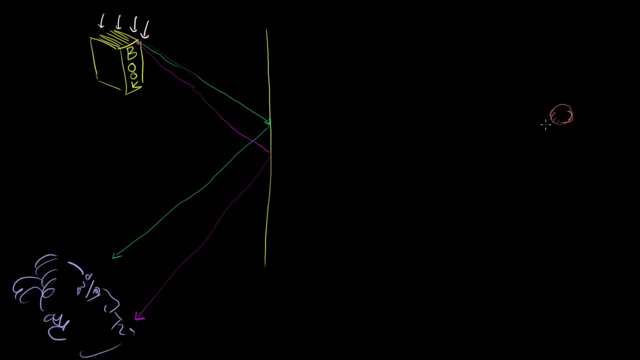 let's say that's an orange right over there. Just ignore all of the stuff on the left. If I were to look at an orange- no mirror, nothing, no reflections or anything. if I were to look at a certain point on the orange, 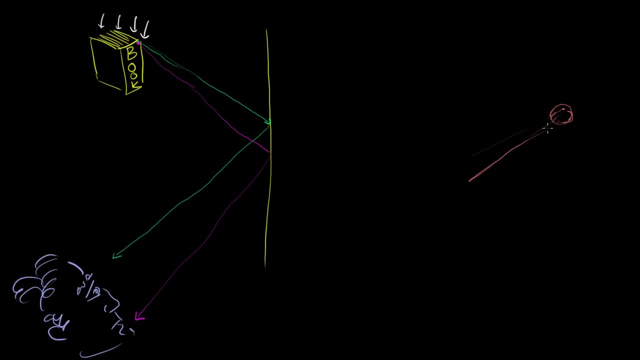 light from that point would be diverging out radially. And if my eye were right over there, my brain says, OK, I have these light rays diverging from a single point. It will simulate or it will show me that point on an orange in my brain. 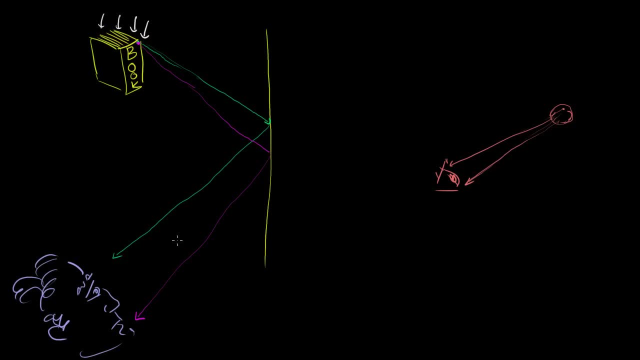 Now the same thing is going to happen here, Even though the light, these two rays actually aren't diverging from a point out here. your brain will say, OK, I've got two things that are coming out. They're coming out from what looks like a point over here. 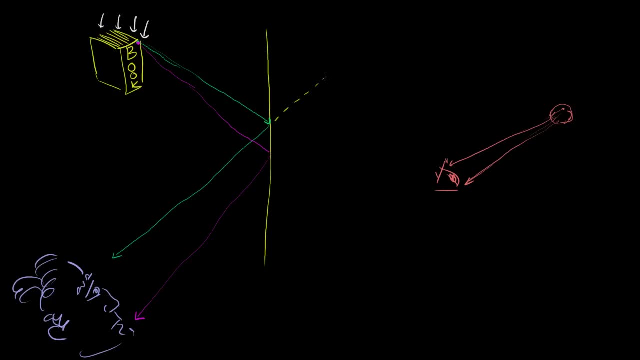 It'll really just extrapolate these lines backwards. So it'll take that green ray and it'll say, OK, it must be coming from a point out there. And it'll take that magenta ray and it'll say it must be coming from a point out there. 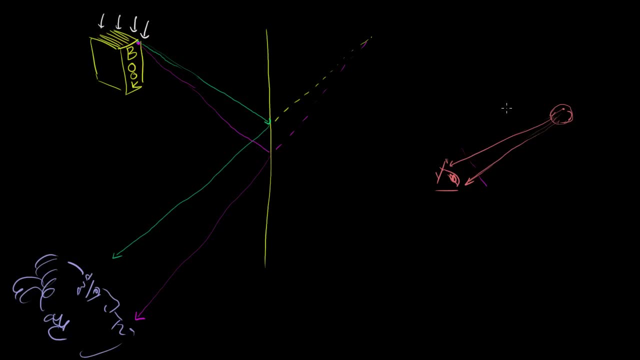 Even here, your eye is just seeing these two light rays. It doesn't know what's going on over here, It just says, OK, they're just converging from a point. And so in this person's reality, or in my reality, 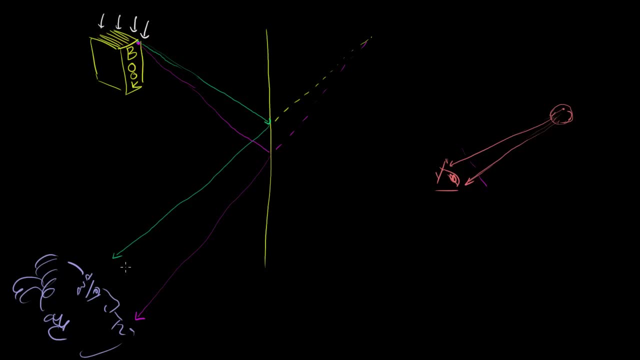 I think that there is an orange there. Likewise, I see these two light rays diverging from some common point. I will extrapolate to figure out, or my brain will try to think about, where that point is in three-dimensional space. It says: look, these two rays look. 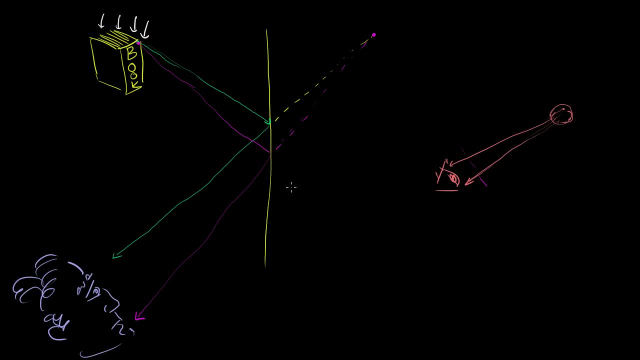 like they're coming from a point back over here. Now the reality is there is no back over here. There is nothing. We're assuming there's nothing behind the mirror, But to this observer it looks like the light is being emitted behind the observer. 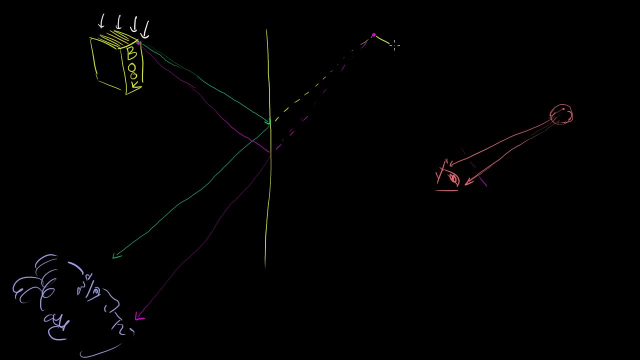 And so what the person would actually see is something like this. The person would actually see something like this, And this is probably not too foreign to any of our experiences. We've all looked in mirrors And remember. this is the right side of the book. 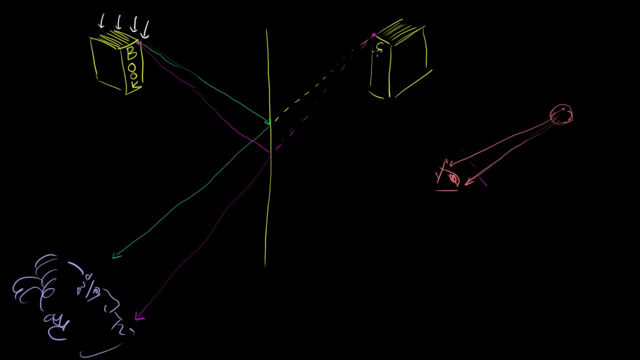 It's the side that has the curvy part of the B. So it's the side that has the curvy part of the B, So it'll look like this. So what this observer sees is an image that looks like this. It is what people call the mirror image. 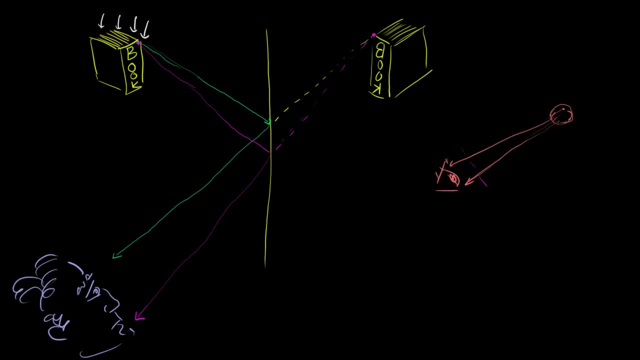 It is flipped. The left and the right is flipped And you can think about why that is. I could just draw another ray right here to make it clear. If this ray is coming like this now, it will reflect and come out back like this: 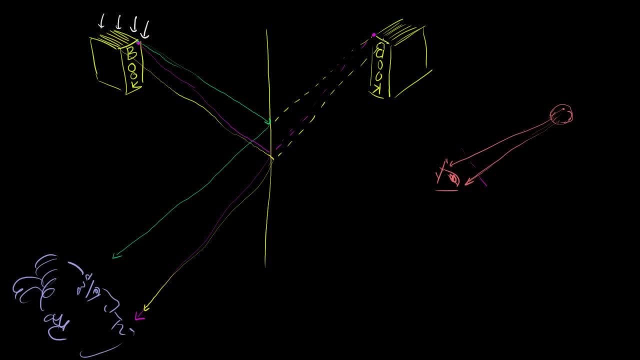 To this observer. it came from that point right over there, So he sees a flipped version of the book. Now, the whole reason why I did this is one: just to make you feel a little comfortable with these reflecting lines, and all of that. 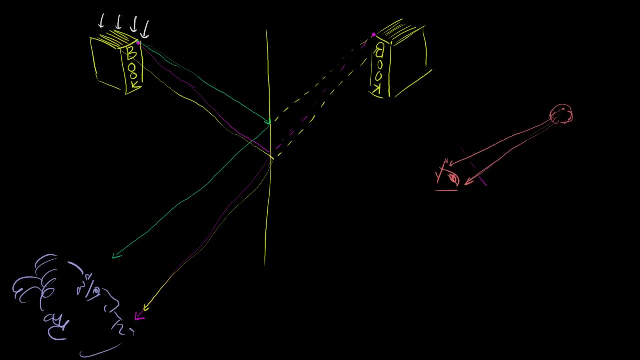 But one, I guess, more importantly, to get you more comfortable, I put the idea of a virtual image This right. here is a virtual image And we're going to compare it with a real image in the next video- And, to some degree, a virtual image. 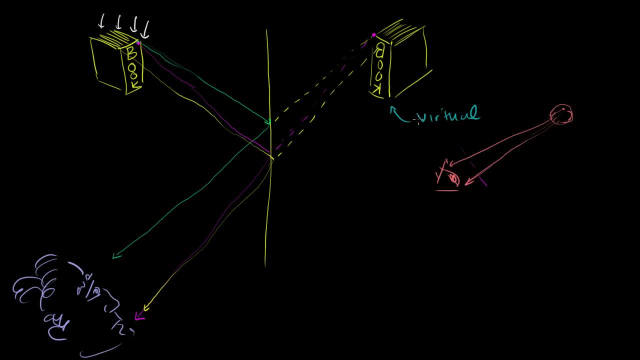 is more intuitive because we have so much experience with it when we think about mirrors or reflected surfaces. So it's a virtual image. And we call it a virtual image because the book really isn't there. It's virtually there. There is no actual physical space. 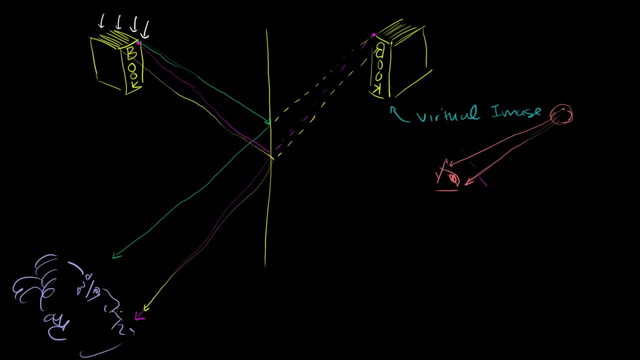 Or we don't know if there's any physical space behind the image. Our brain just uses these diverging lights and creates a model inside of our brain or whatever, to say: OK, that book exists there, even though the source of the light is over here. 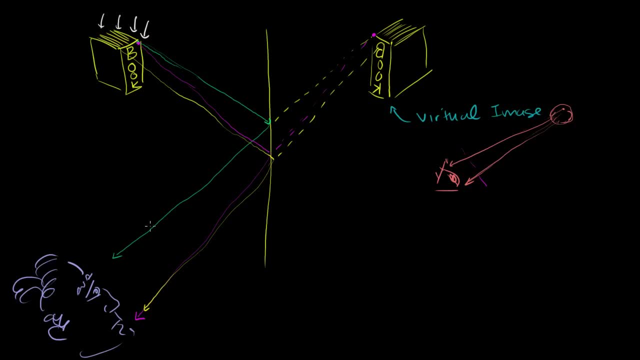 Now I'm just going to draw another diagram, And this is more. you know you normally won't have the diagrams that have this type of perspective, But just to give you a sense of the same thing and just to get you familiar with some of these diagrams, 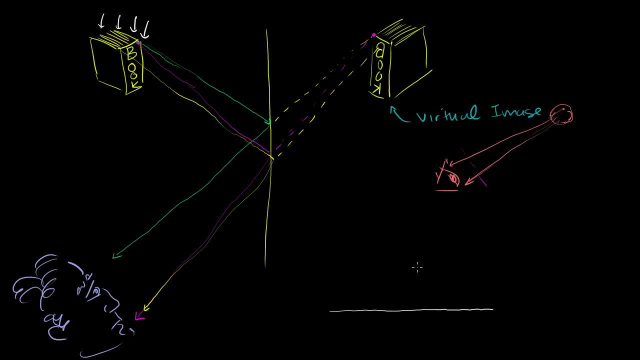 we're going to do when we study mirrors and lenses is we could imagine that. let's say that this is the ground, Let's say that this is a mirror And let's say that this actually could be somebody standing in front of a mirror. 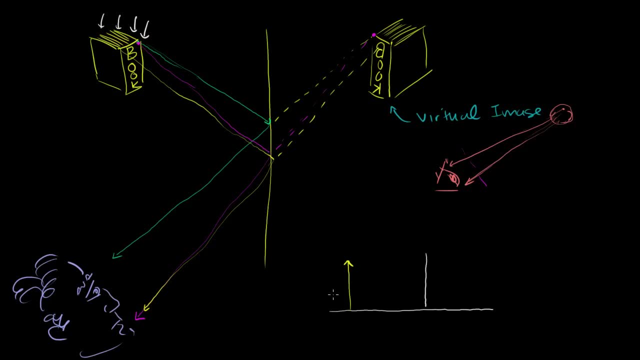 Although usually people will draw an arrow here to just say an arbitrary object. Well, let's just say we have an arrow in front of the mirror, just so you get used to this notation. This is actually a physical arrow, This is not a light ray. 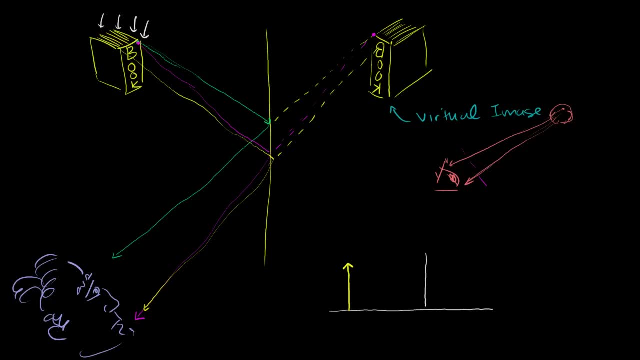 Now let's think about what the image of this arrow? Let's say this arrow had eyes, so it's actually a person. So this arrow had eyes. What would this arrow see? Well, let's just pick an arbitrary point on this arrow. 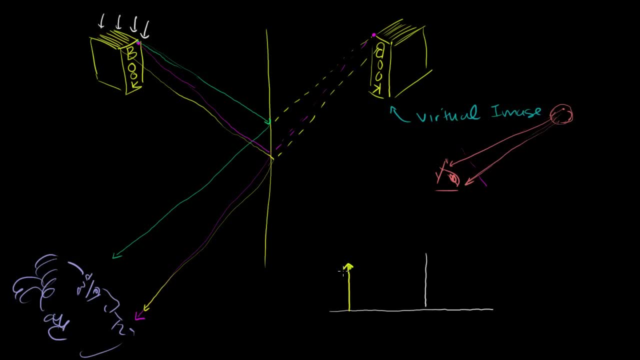 You could do it with any point with this object, because every point will be reflecting light diffusely. So I'm going to take one point that's coming straight out of the mirror, one light ray that goes straight to the mirror, so just parallel to the ground. 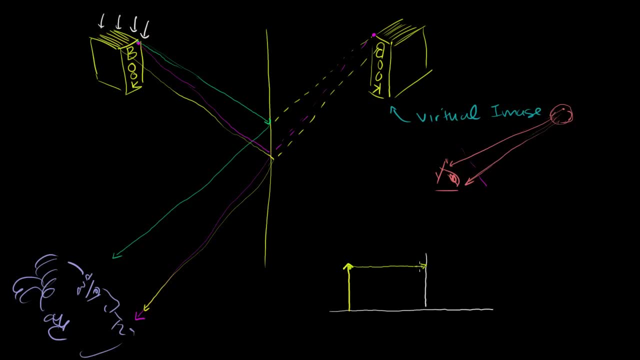 straight to the mirror. Well, it's just going to reflect straight off and then come back. It's just going to go straight off and then come back to the source of that light, maybe that arrow's eye if you view it as a person. 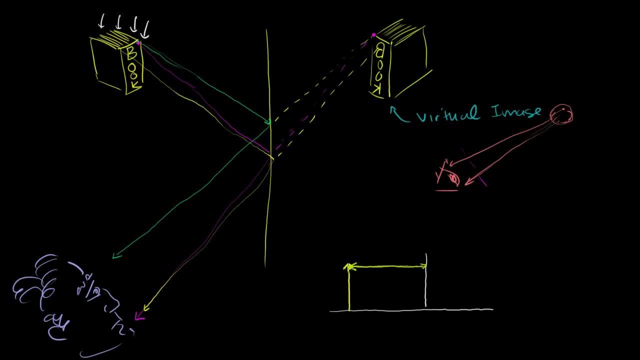 And let's just do another point, another ray coming from that point, So another ray coming from that point might come out like that: Incident angle is equal to reflected angle. so then it would come back like that. Now, maybe this whole thing is an eye.